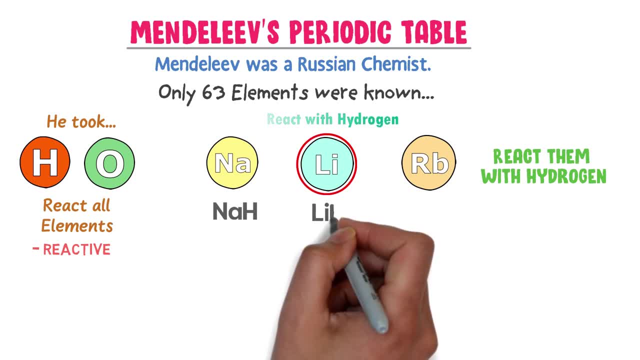 When lithium reacts with hydrogen, it forms lithium hydride, And when rubidium reacts with hydrogen, it forms rubidium, hydride, Sodium, lithium and rubidium. Sodium and rubidium form same type of compounds with hydrogen. 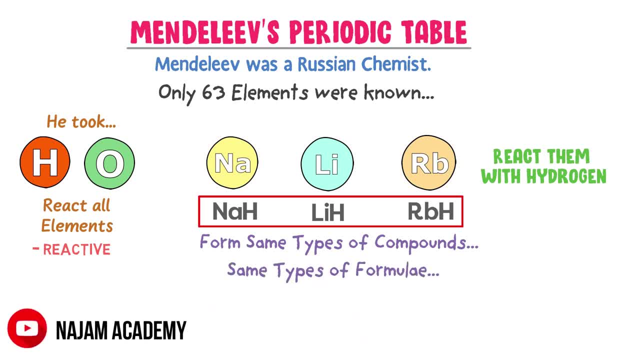 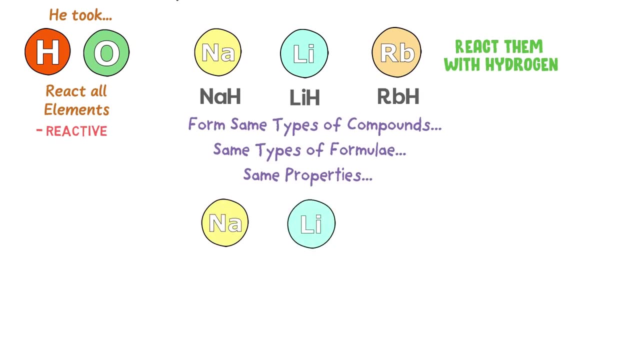 They have same formula of hydrides, For example, one to one ratio. Also, all these compounds have same properties. For example, all these compounds are soluble in the water. Secondly, he again took sodium, lithium and rubidium and reacted them with oxygen. 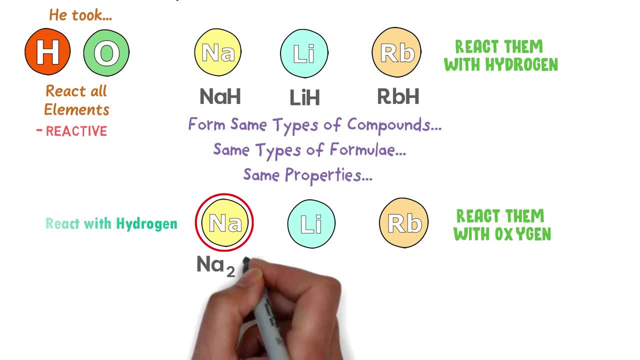 When sodium reacts with oxygen, it forms sodium oxide. When lithium reacts with oxygen, it forms lithium oxide. And when rubidium reacts with oxygen, it forms rubidium oxide. So the oxides of sodium, lithium and rubidium also have same formula. 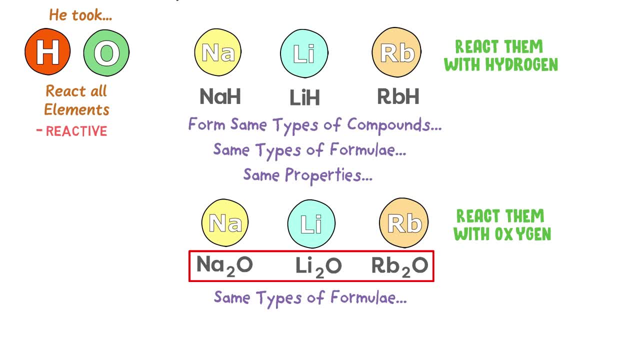 For example, two ratio to one. Also, these oxides have same properties. For example, these all compounds are basic compounds, Hence Mendeleev baba. abhisa Mendeleev baba observed that sodium, lithium and rubidium form same type of hydrides and 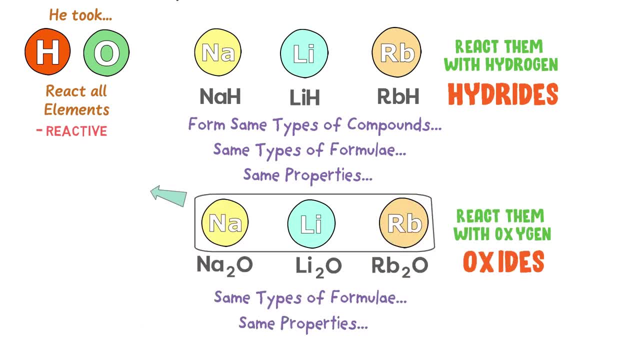 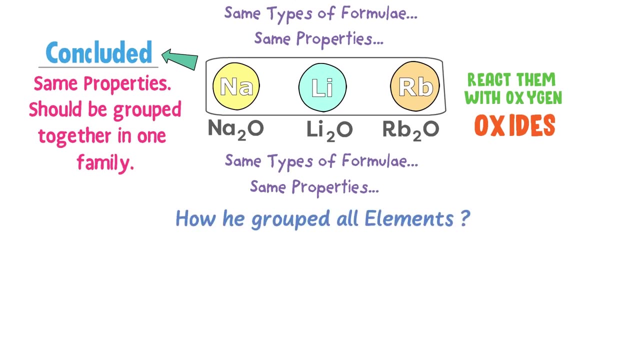 oxides. Their compounds have same properties. So he concluded that sodium, lithium and rubidium have also same properties, Or these three elements should be grouped together in one family. Now how he grouped all elements? Well, he arranged elements according to atomic masses. 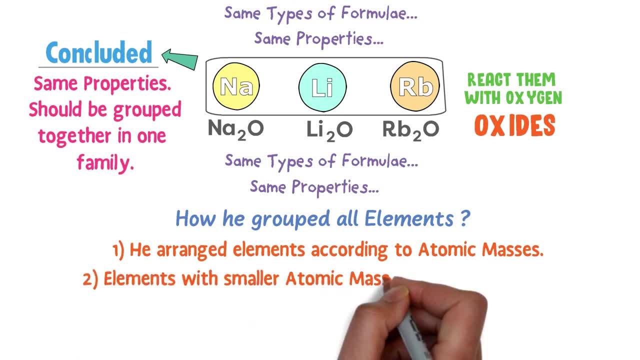 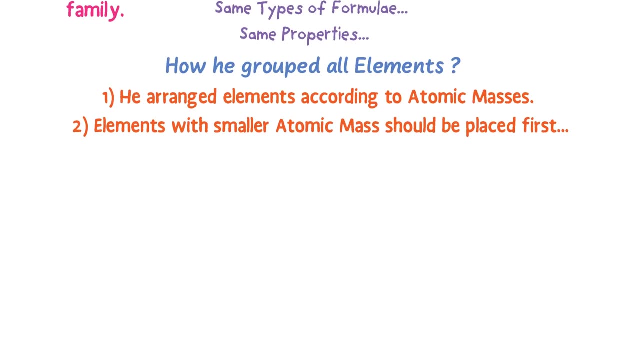 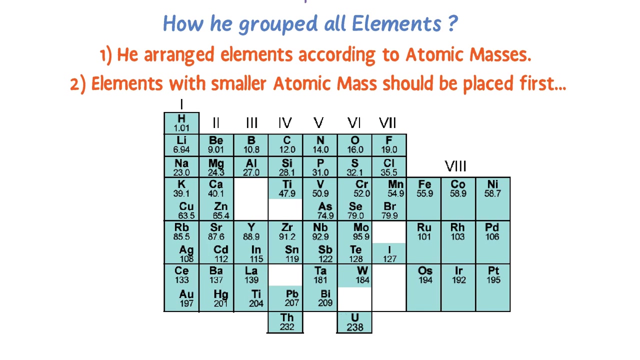 He stated that elements with smaller atomic mass should be placed first and elements with greater atomic mass should be placed second. Thus, remember these two properties of Mendeleev's periodic table. He arranged all elements in eight columns and ascending order of atomic masses, called groups. 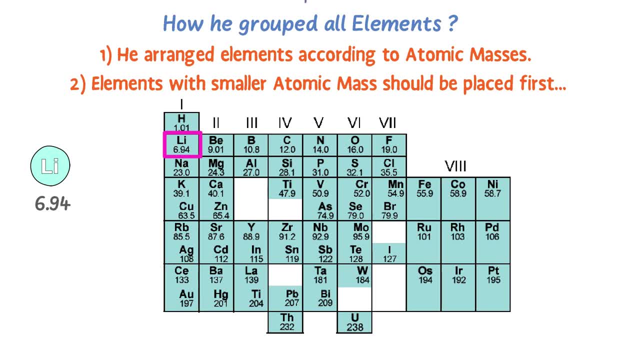 For example, the atomic mass of lithium is 6.94.. The atomic mass of hydrogen is 6.94.. The atomic mass of hydrogen is 6.94.. The atomic mass of hydrogen is 6.94.. The atomic mass of beryllium is 9.01.. 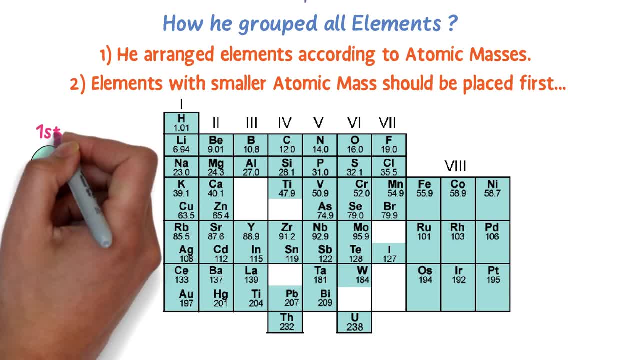 The atomic mass of beryllium is greater than lithium, so beryllium is placed after the lithium. Secondly, every group contains elements having same properties. For example, all the elements in group 1 have same properties. All the elements in group 5 have same properties. 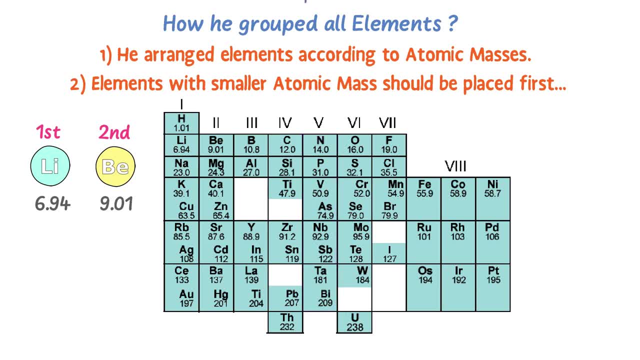 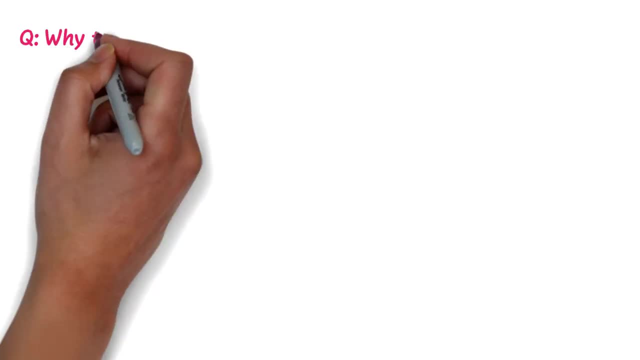 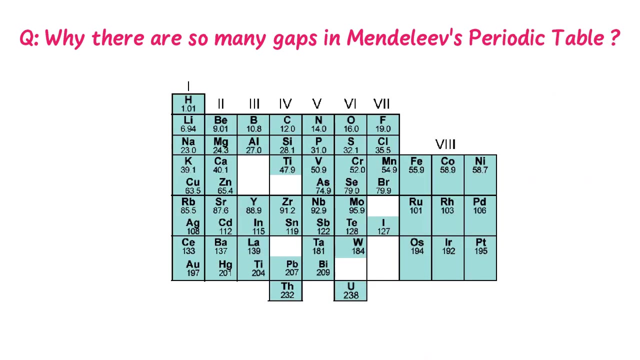 Thus remember that Mendeleev arranged all elements on the basis of atomic mass. Now let me teach you some conceptual questions. Why did Mendeleev arrange the periodic table with so many gaps in it? Well, he ensured that in every group, all elements should be placed with same properties. 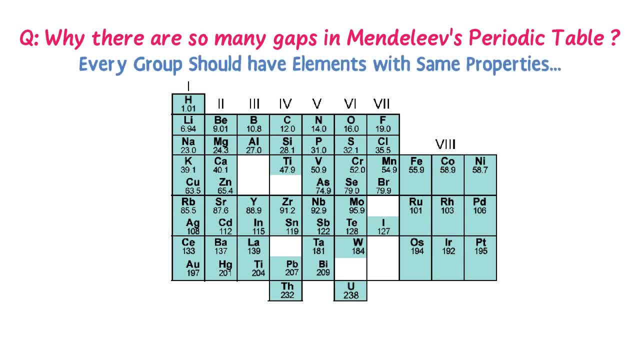 Now, when he first Whenhhharrange at arsenic, he wanted to put to put theAR feature on it. So you have toелен danced, be, danced when, when. 냉 next x now m I w dust, m m below aluminium, But wait a minute. He observed that the properties of arsenic are different from 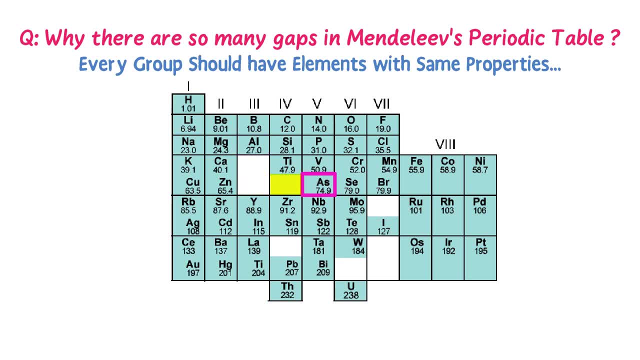 aluminium, So he left a gap. Secondly, he wanted to place arsenic below titanium, But he observed that arsenic has also different properties than titanium, So he again left a gap. Finally, he placed arsenic below phosphorus and vanadium. He observed that arsenic has same properties as 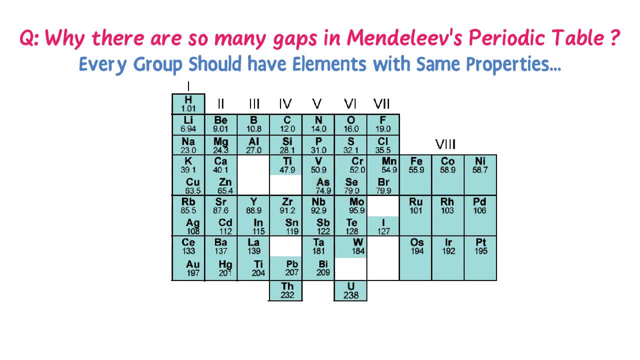 phosphorus or vanadium has. Also, Mendeleev Baba was so genius that he stated these gaps exist because we haven't yet discovered these elements. Even he predicted the properties of these not yet discovered elements. Mendeleev called these unknown elements as acaburon. 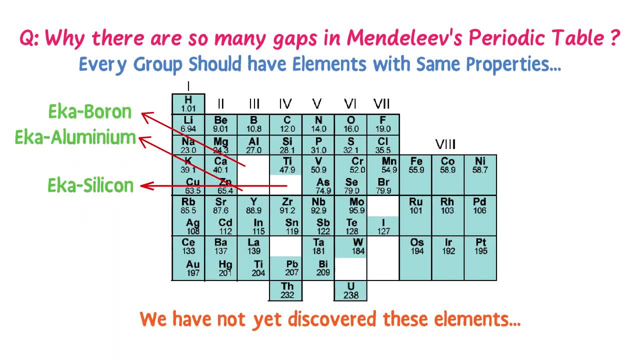 eka-aluminium and eka-silicon. Later we discovered all these three elements as scandium, gallium and germanium. These three elements almost match the properties of Mendeleev. Thus note it down that Mendeleev left gaps in his periodic table because all these elements